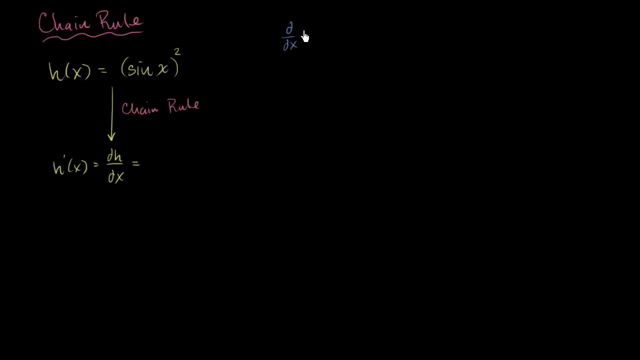 If I were to ask you what is the derivative with respect to x, If I were to supply the derivative operator to x squared, I would have to do the following. I would have to do the following: If I were to take the derivative with respect to x, squared with respect to x, what do I get? 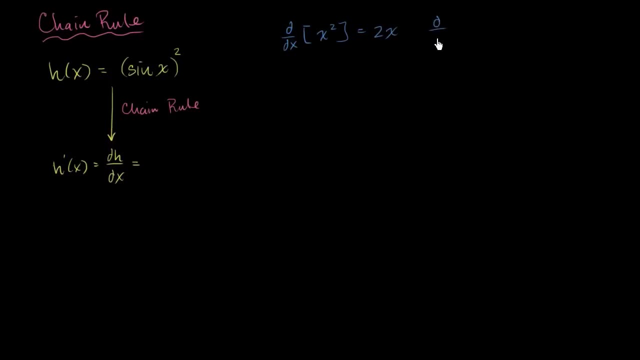 Well, this gives me 2x. We've seen that many, many, many, many times. Now, what if I were to take the derivative with respect to a of a squared? Well, it's the exact same thing. I just swapped an a for the x's. 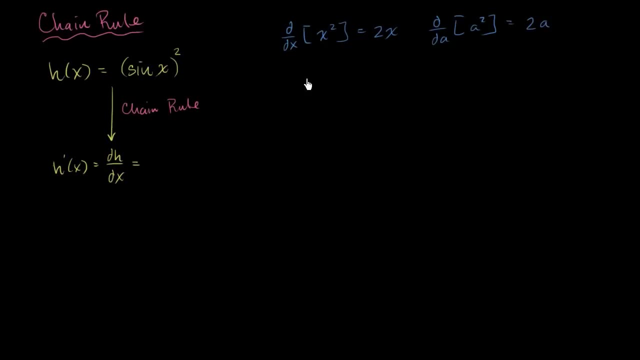 This is still going to be equal to 2a. Now I will do something that might be a little bit more bizarre. What if I were to take the derivative with respect to sine of x, of sine of x squared Well, wherever I had the x's up here? 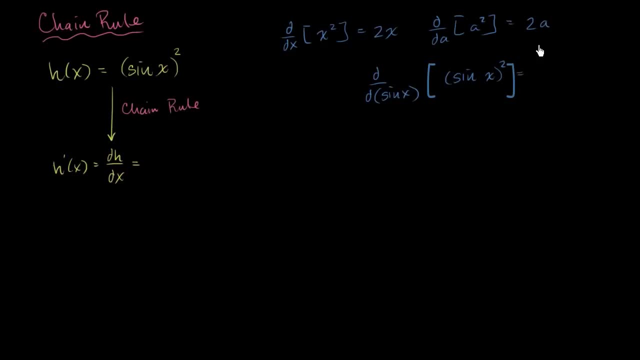 or the a's over here. I just replaced it with a sine of x, So this is just going to be 2 times the thing that I had. So, whatever, I'm taking the derivative with respect to Here, with respect to x, here, with respect to a, here, with respect to sine of x. 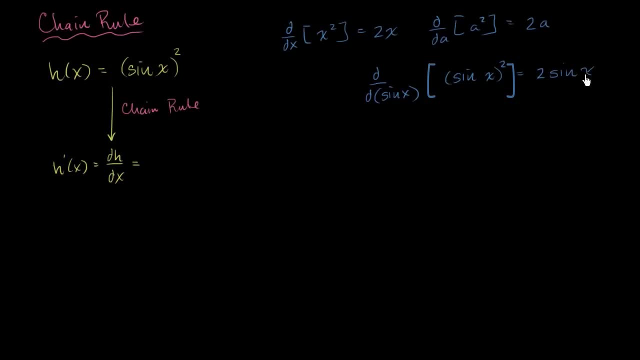 So it's going to be 2 times sine of x Now. so the chain rule tells us that this derivative is going to be the derivative of our whole function with respect, or the derivative of this outer function: x squared. The derivative of x squared. the derivative of this outer function with respect. 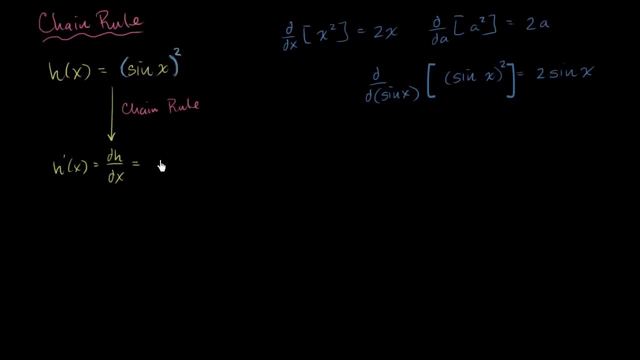 to sine of x. So that's going to be 2 sine of x. 2 sine of x, So we could view it as the derivative of the outer function with respect to the inner 2 sine of x. We could just treat sine of x like it's kind of an x and it would have been just 2x. 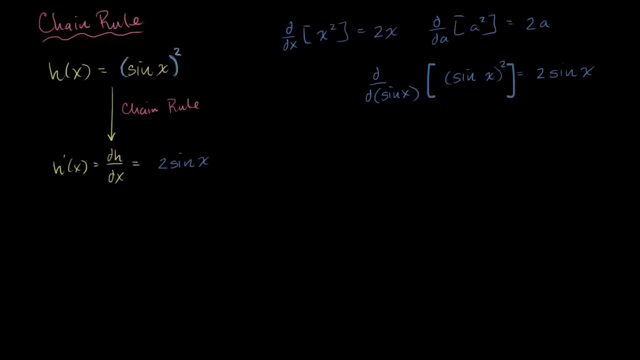 but instead it's a sine of x. So we say 2 sine of x times times the derivative. Let me do this in green Times: the derivative of sine of x with respect to x Times the derivative of sine of x with respect to x. Well, that's more straight forward, or a little bit more. 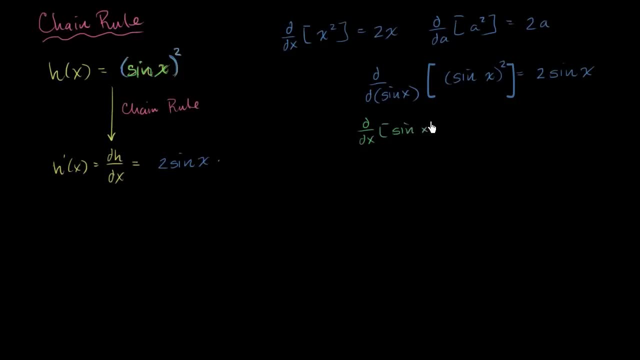 intuitive. The derivative of sine of x with respect to x- we've seen multiple times- is cosine of x, So times cosine of x. And so there we've applied the chain rule. It was the derivative of the outer function with respect to the inner, So derivative of sine of x. 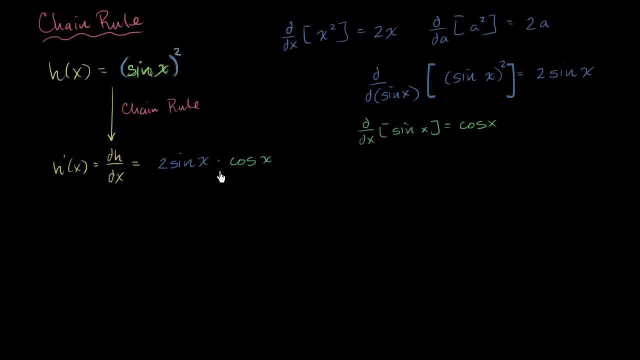 squared with respect to sine of x is 2 sine of x, And then we multiply, that times the derivative of sine of x with respect to x. So let me make it clear This right over. here is the derivative. We're taking the derivative of. 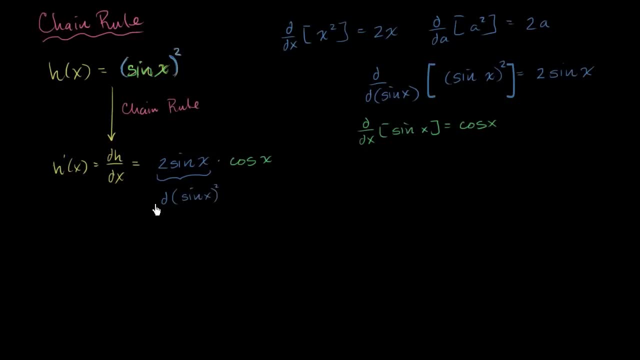 sine of x squared. So let me make it clear: That's what we're taking, the derivative of, with respect to sine of x, With respect to sine of x, And then we're multiplying that times the derivative of sine of x, The derivative of sine of x with respect. 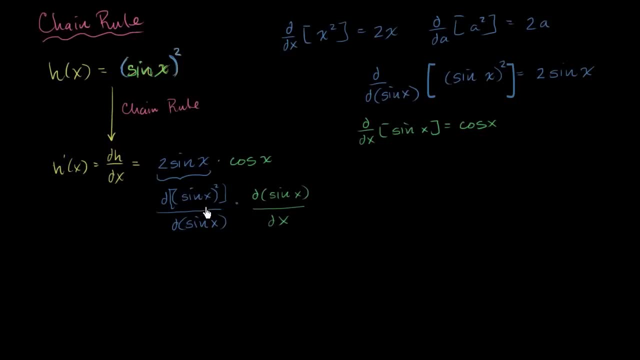 to x. And this is where it might start making a little bit of intuition. You can't really treat these differentials, this d, whatever, this dx, this d sine of x, as a number, And you really can't. The notation makes it look like a fraction- because, intuitively, 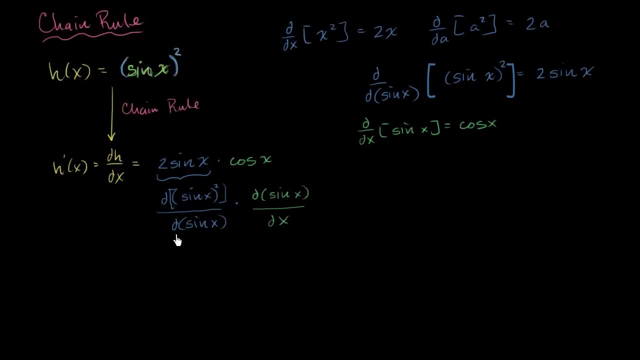 that's what we're doing, But if you were to treat them like fractions, then you could think about canceling that and that- And once again, this isn't a rigorous thing to do, but it can help with the intuition- And then what you're left with is the derivative of 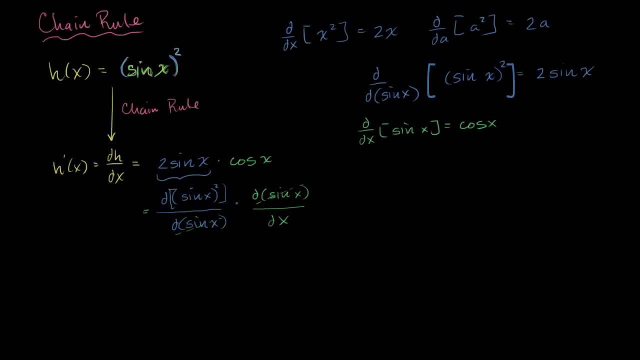 this whole sine of x squared with respect to x. So you're left with the derivative of essentially our original function: sine of x squared with respect to x, Which is exactly what dh dx is. This right over here is our original function h. 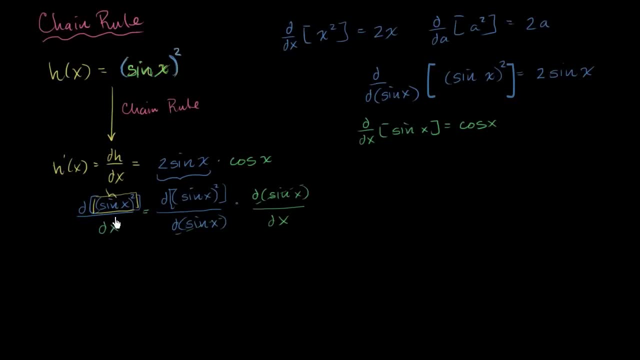 That's our original function h, So it might seem a little bit daunting now. What I'll do in the next video is another several examples, and then we'll try to abstract this a little bit.